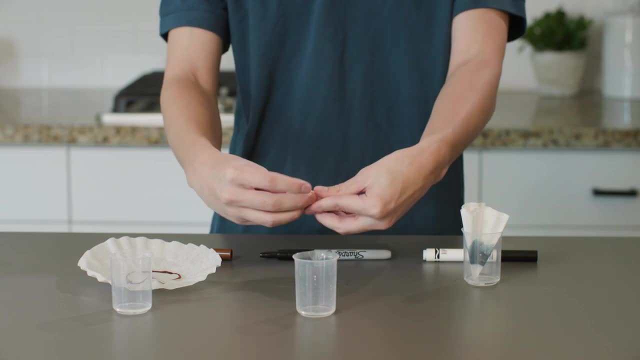 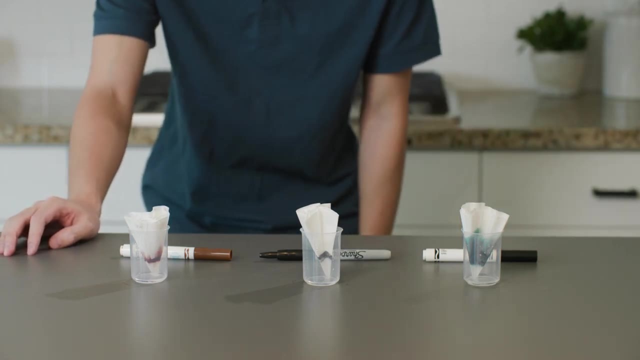 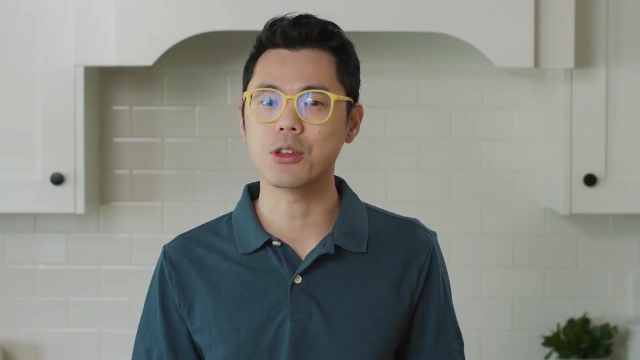 Okay, now let's put each filter point down into the water. Look at that: The color is already starting to separate in some of the cups. Okay, we have to wait for about seven minutes to allow the water to spread up through the coffee filter and through the ink. 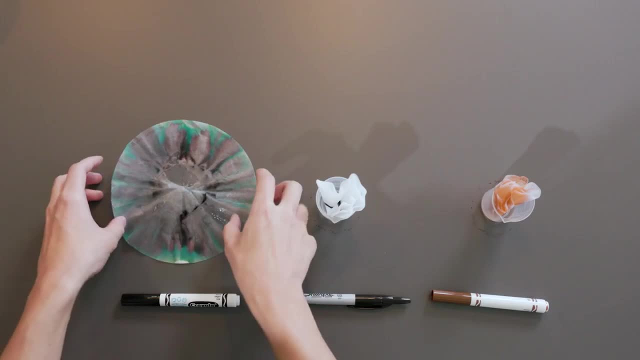 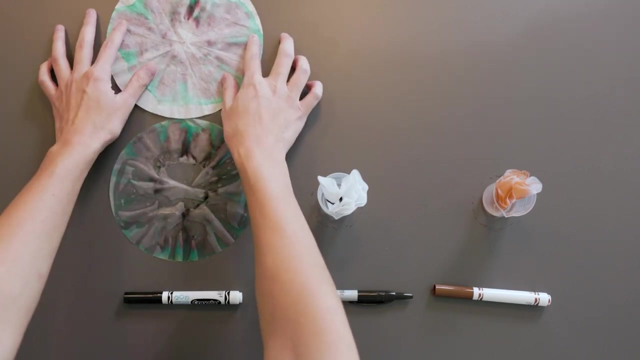 Are you ready to see what happened to each color? This is the black washable marker. Do you see the different colors? Okay, here is another coffee filter that I prepared earlier. This one is completely dry. Can you see any colors in the dry filter that you can't see in the wet one? 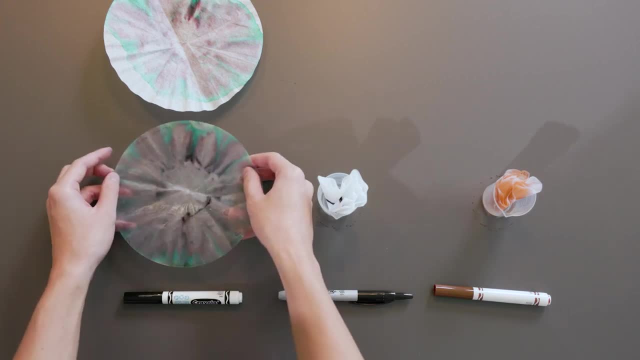 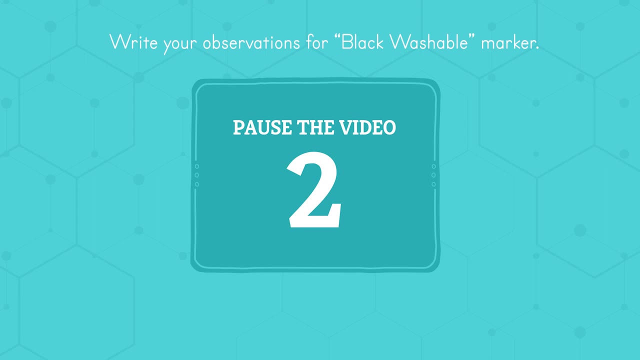 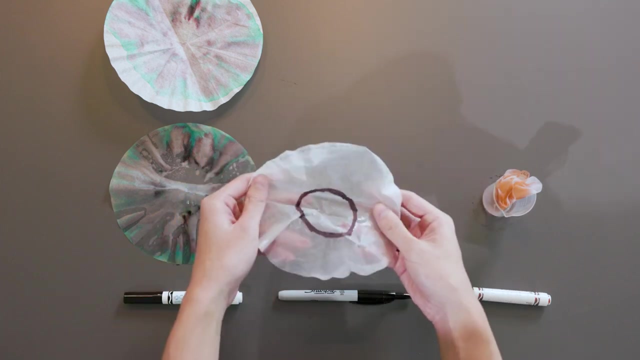 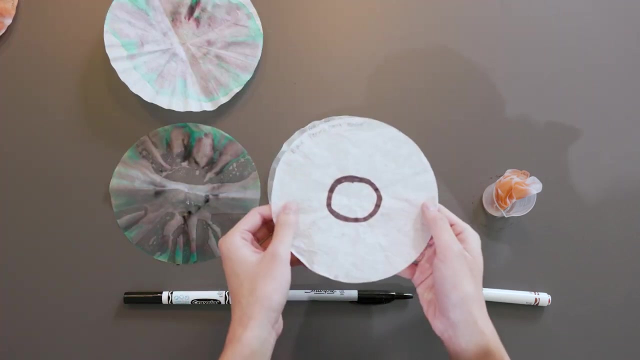 Pause the video now and write down your observations in the results section of your student journal. for the black washable marker: Okay, let's look at the black permanent marker now. Hmm, that's interesting, This one didn't separate at all. Let's look at this completely dry filter that I prepared earlier. 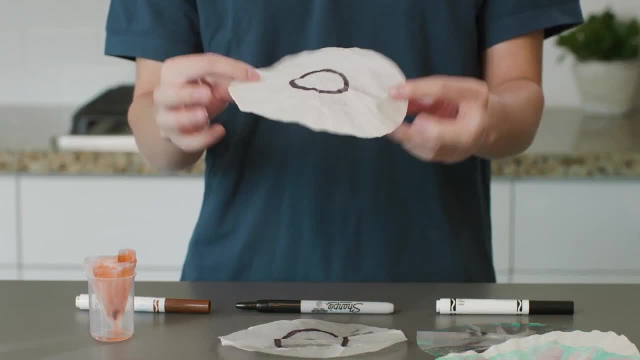 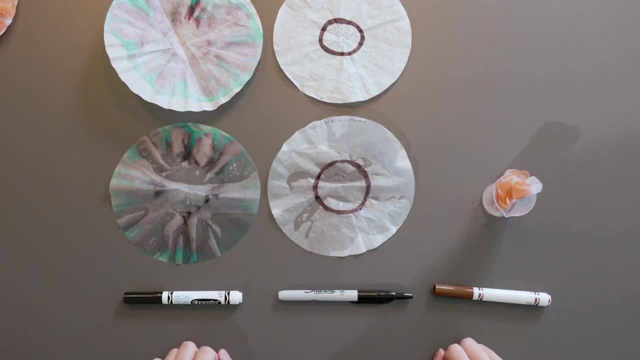 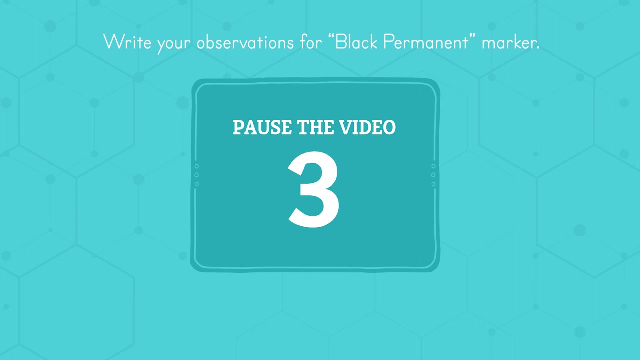 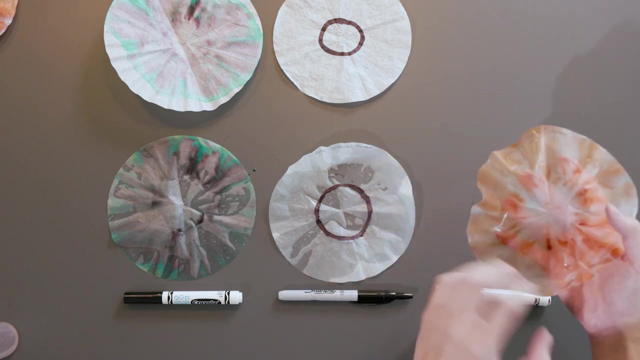 This one did not separate at all either. Why do you think that happened? Permanent markers are not water soluble, meaning the ink does not dissolve with water. Go ahead and pause the video and record your observations of the black permanent marker, Alright. finally, let's check out the brown washable marker. 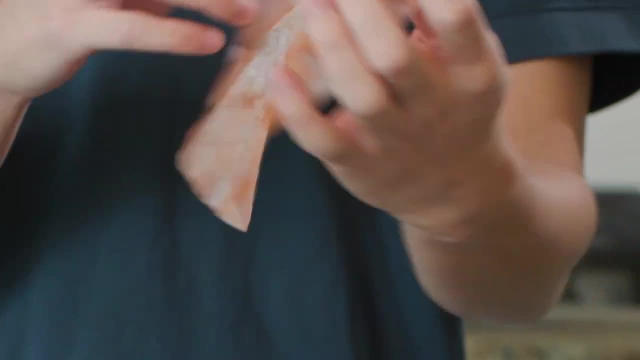 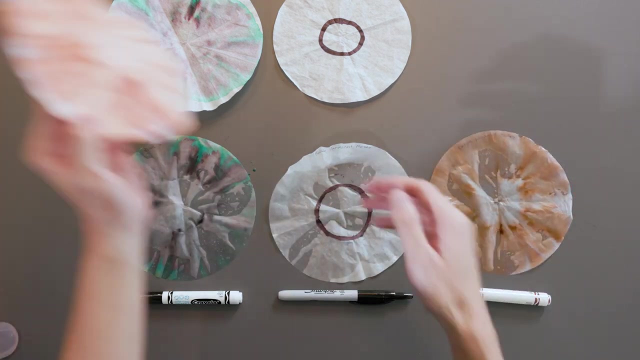 This one is interesting. It's not as easy to see the color separation here as it was for the black marker. What colors can you see? Maybe it will be easier to see the color separation in the dry one I prepared earlier. Can you see the color right on the edges of this one? 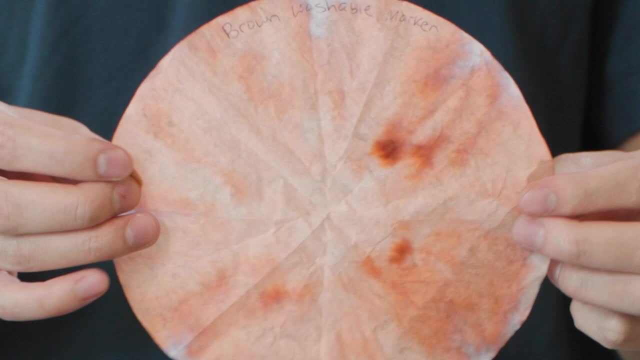 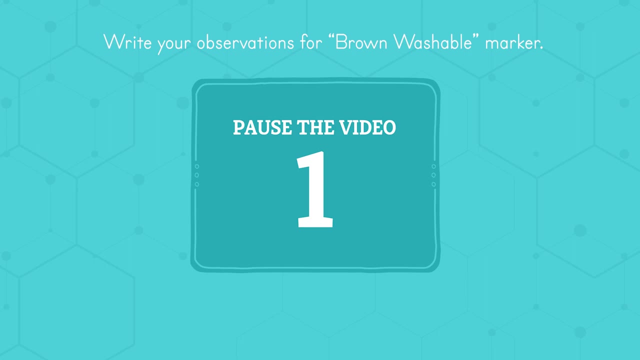 Pause the video now and record your observations of the brown washable marker. Can you see the color right on the edges of this one? Maybe it will be easier to see the color separation in the dry one I prepared earlier. If you try this experiment at home, consider trying other colors of markers. 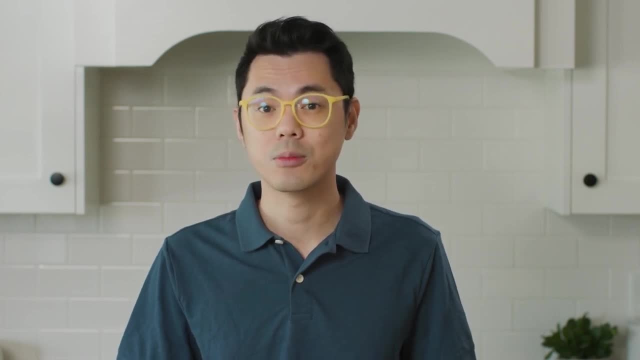 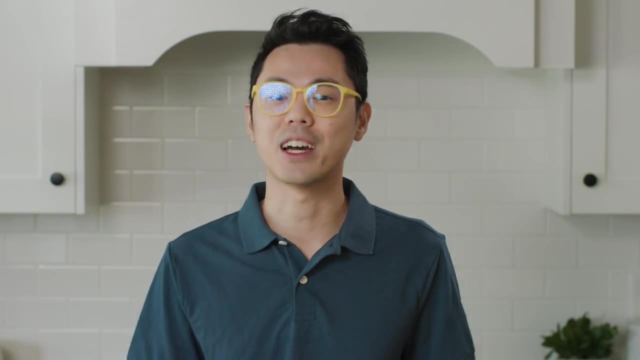 or consider using a different solution. besides water, Permanent markers are not water soluble, but what would happen if you used oil or rubbing alcohol instead? Try it and find out.